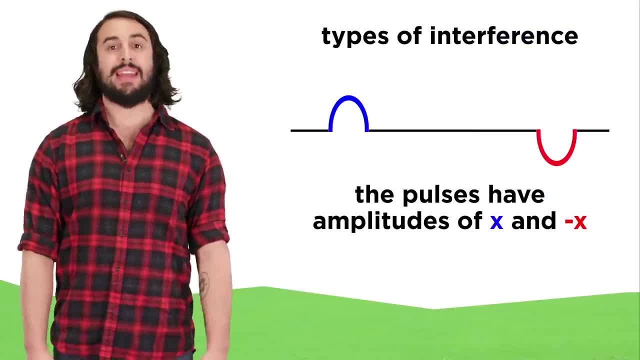 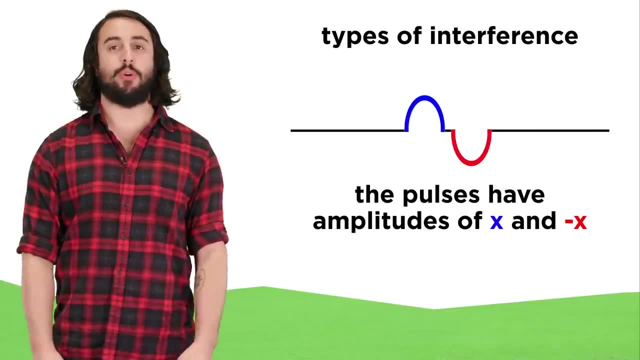 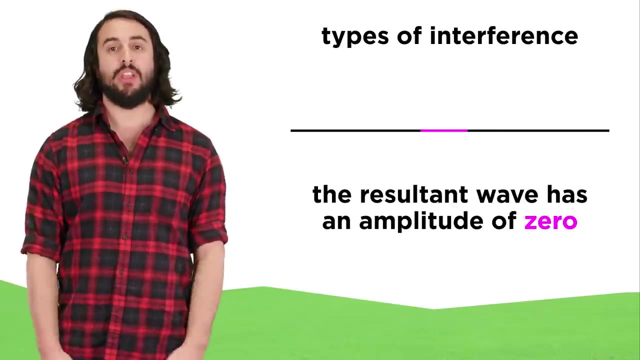 this is called constructive interference. Now let's say the pulses are on opposite sides of the equilibrium position. Again, according to the superposition principle, we will add the amplitudes to get the resultant wave. but in this case the two amplitudes add to zero, so the resultant wave will be: 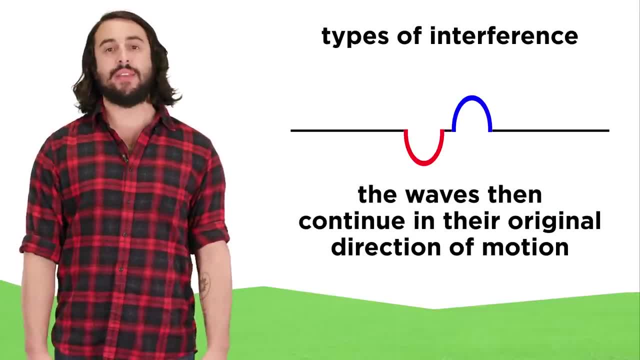 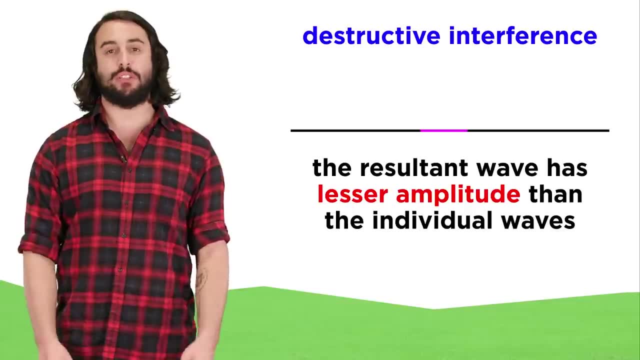 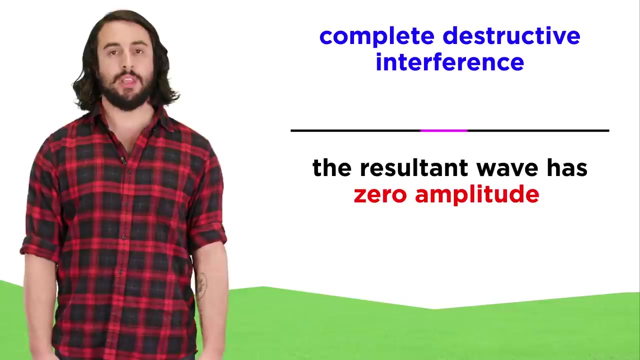 as though there is no wave at all. Then the waves continue along their trajectories. This kind of interference, where the resultant wave has a smaller amplitude than the individual waves, is called destructive interference, and if the resultant wave has an amplitude of zero, like this example, it is called complete destructive interference. 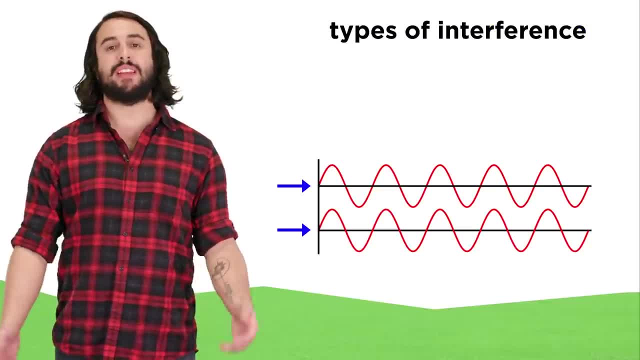 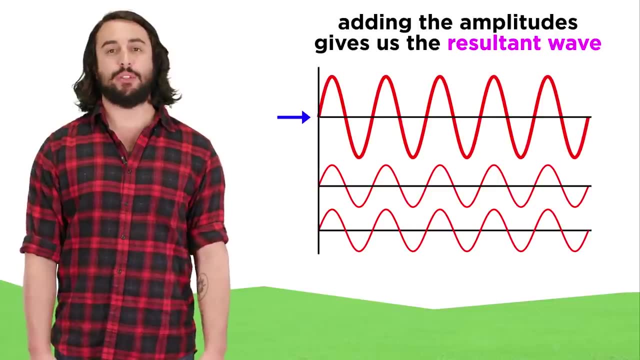 This concept applies to periodic waves as well. First, we can consider two sine waves that are precisely aligned. They are said to be exactly in phase. We can add the amplitudes at every single point and the result is a similar looking wave with twice the amplitude due to constructive interference, because the crests align with. 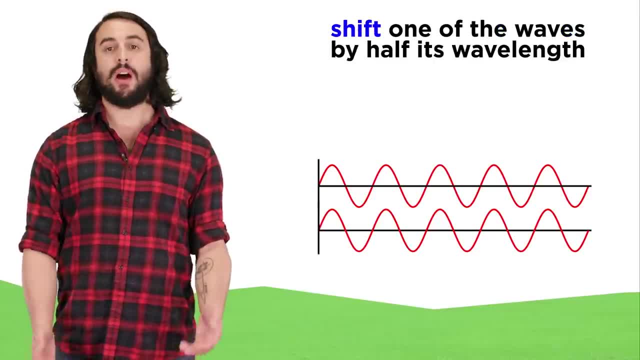 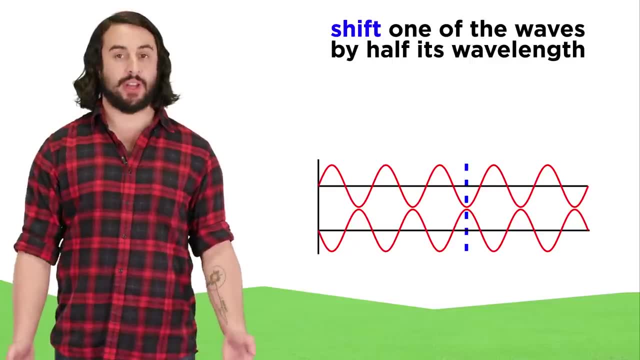 the crests and the troughs align with the troughs, But then if we shift one of these by half its wavelength, now the crests of one align with the troughs of another and at every single point on the x-axis these waves will. 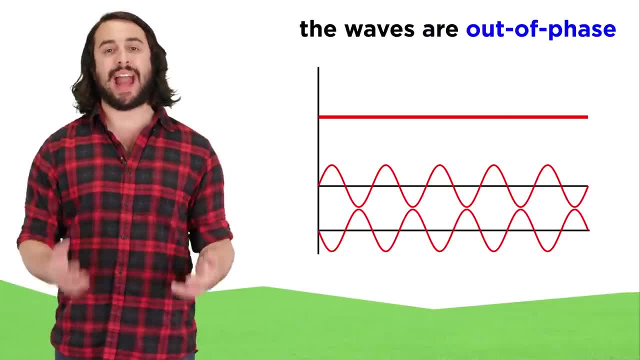 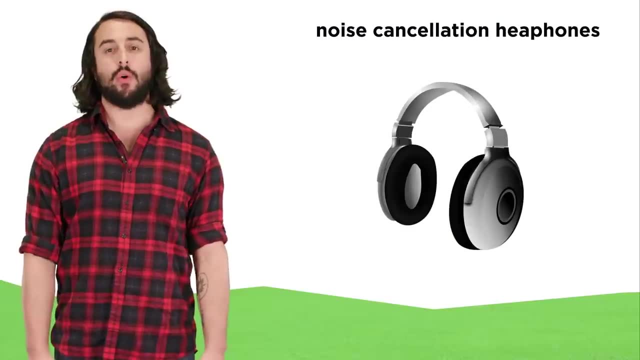 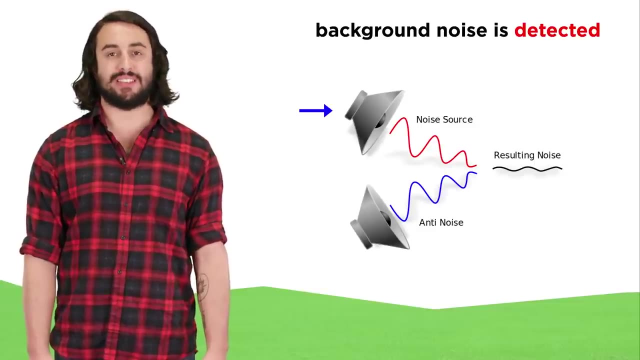 add up to zero, They are said to be exactly out of phase, and this will be an example of complete destructive interference. This is what noise cancellation headphones do. Small microphones detect background noise and process the associated signal and then reproduce this noise in a way that is precisely out of phase with the signal. 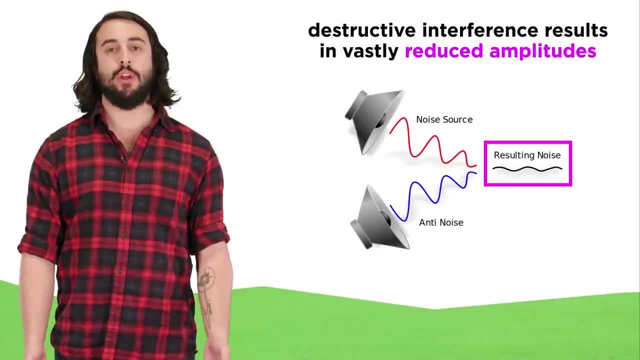 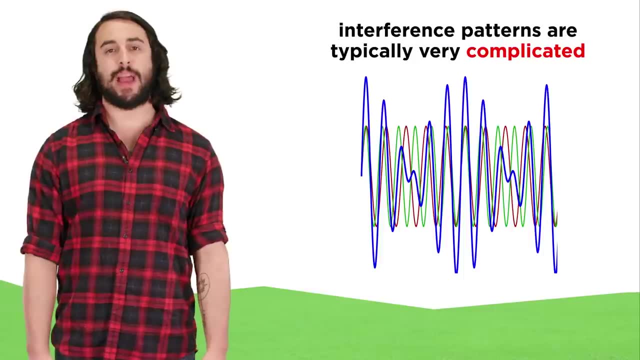 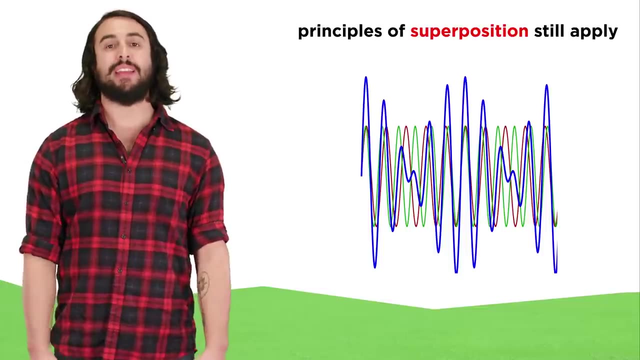 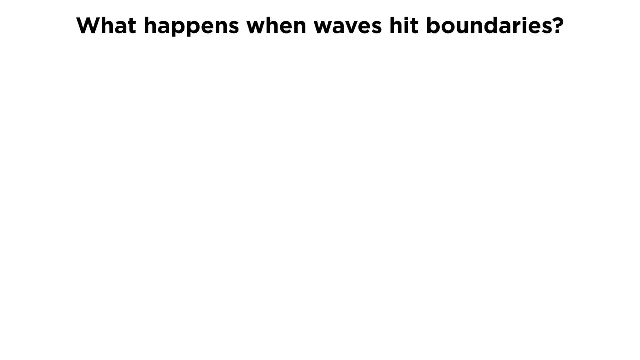 The resulting destructive interference results in zero, or at least dramatically reduced, sound waves reaching urea. In reality, interference patterns are often much more complicated than these two extremes, but in every case the superposition principle is still applicable. We also want to understand what happens when waves hit a boundary of some kind. 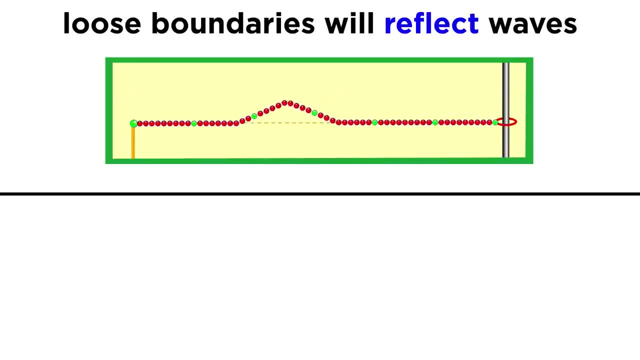 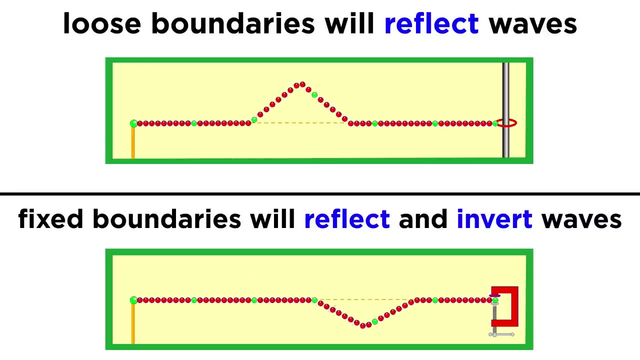 If a boundary is free to move, waves will be reflected, bouncing back in the opposite direction, but maintaining the same amplitude. If, instead, this boundary is fixed, waves will be both reflected and reflected in the opposite direction, but maintaining the same amplitude.